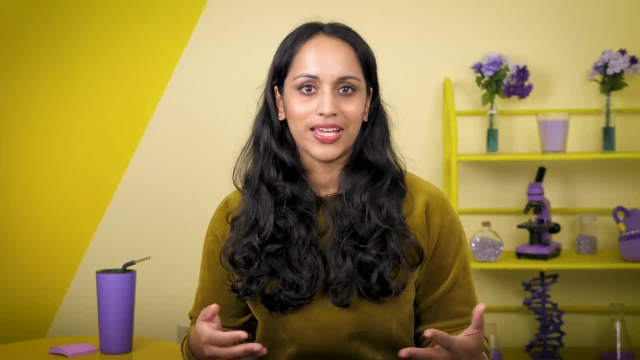 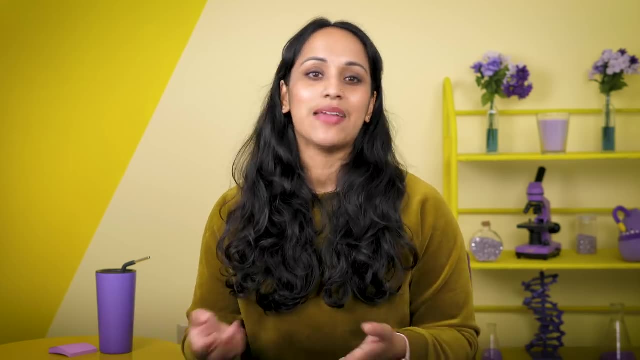 Other scientists have speculated that Kekulé chose to describe his revelation as a dream to avoid sharing credit with his colleagues. Perhaps that's true, but for now it's his name that we find in textbooks. In any case, I'm not here to debate science history, so 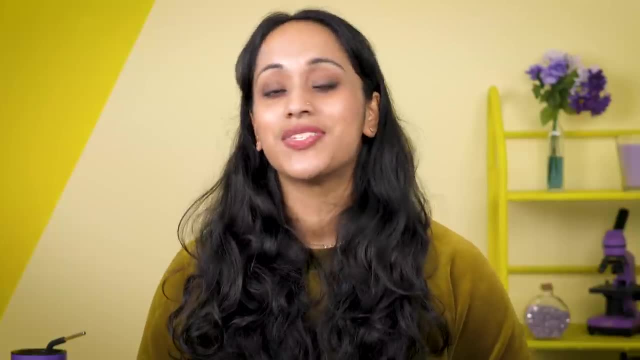 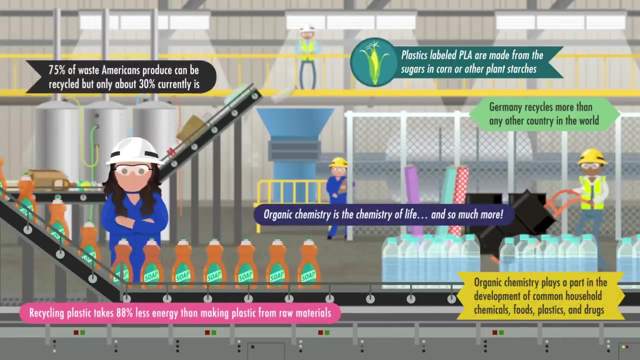 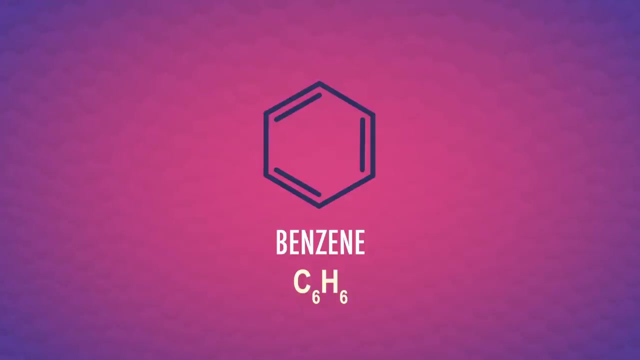 let's take a look at what makes benzene and other aromatic compounds so special. INTRO: Benzene is drawn in a couple different ways. We can think of it with alternating single and double bonds, or we can imagine the pi bond smeared across the whole molecule. 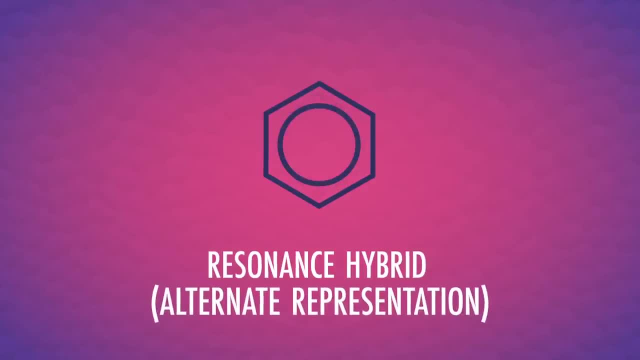 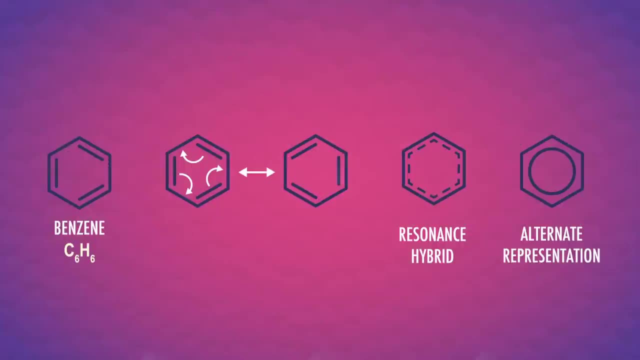 and represent that resonance, hybrid with a dotted line or a circle in the middle. As the statistician George Box famously said, all models are wrong, but some are useful, And that's definitely the case here. Neither diagram is completely right or completely wrong. 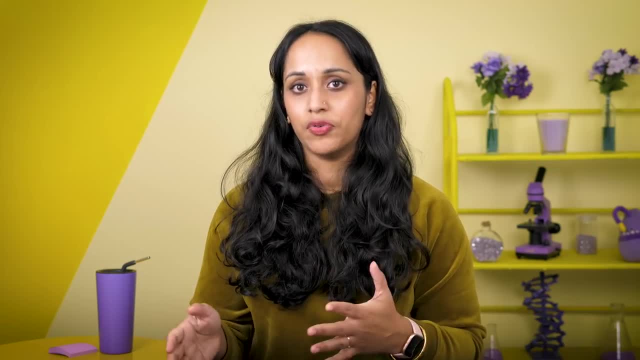 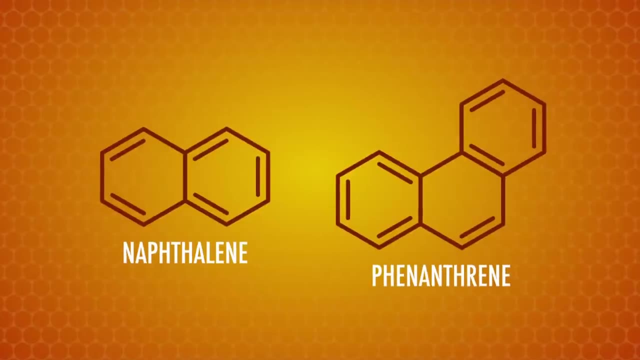 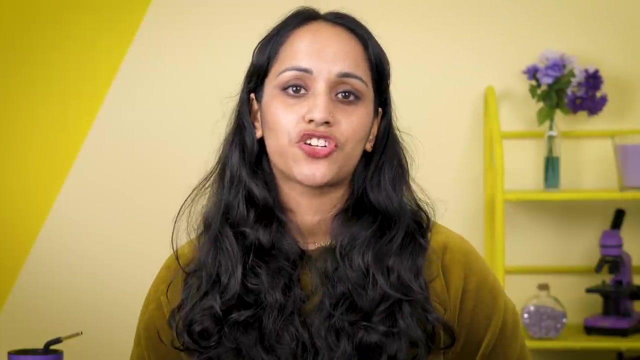 but both have their uses. The alternating bonds version is helpful when we're trying to show which way electrons move in mechanisms. It's also better if we're trying to draw polycyclic aromatic hydrocarbons molecules with joined up aromatic rings. On the other hand, the smeared version more accurately represents the electron. 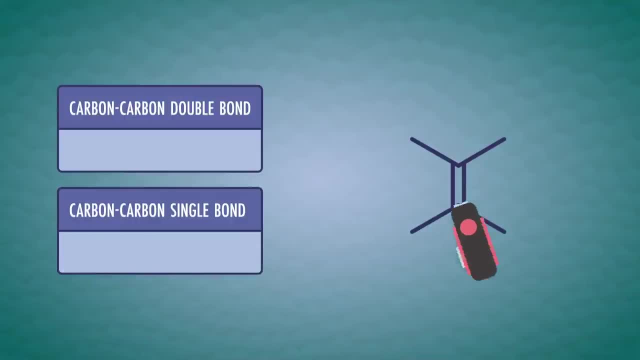 distribution in the benzene ring. You see carbonyl and carbon. double bonds are typically 0.134 nanometers long, while single bonds are 8 degrees N. bah ardi Yoon's studying pistTerra fish, which is a Hepta ion, but also ign voted at прив helplessness. carbon. carbon double bonds are typically 0.134 nanometers long, while single bonds are 0.134 nm long long, while single carbon bonds are slightly longer. So if you drew out Kekulé's model, you'd expect a sort of distorted hexagon. 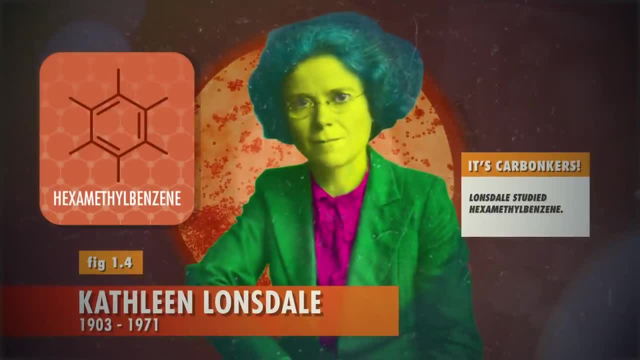 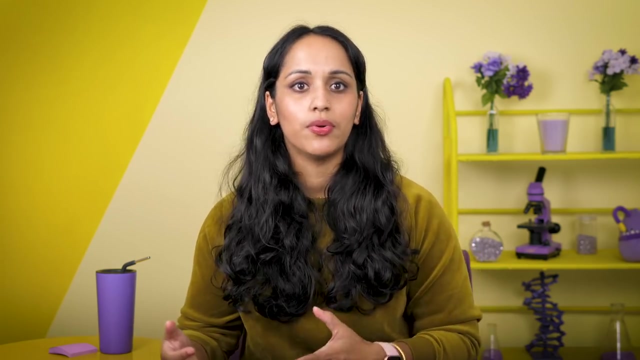 But in a famous paper published in 1929, the English crystallographer Kathleen Lonsdale showed that benzene rings are flat, symmetrical around a central point and the bonds were all the same length. Plus, in chemical reactions benzene doesn't react like an alkene, with some double and 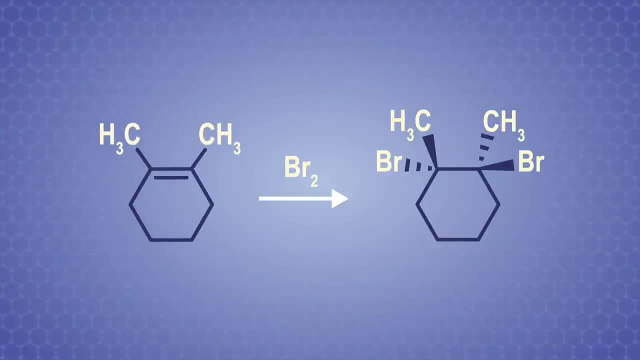 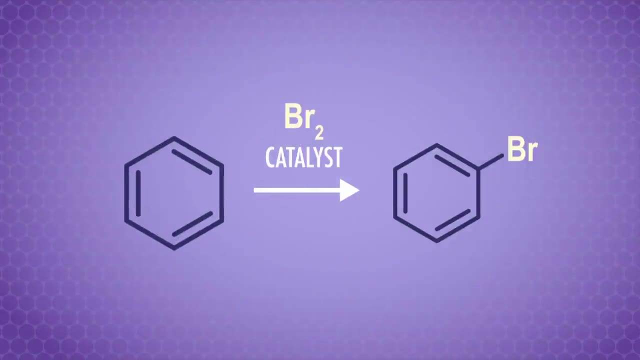 single carbon bonds, For example alkenes, react easily with molecular bromine. The bromines add with anti-addition across the double bond. This doesn't happen with benzene. We need harsher conditions or a catalyst to make anything happen. 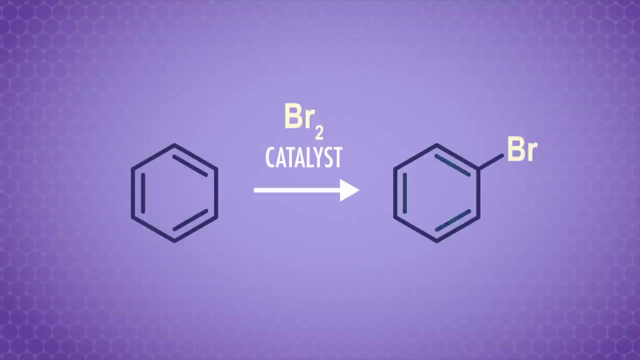 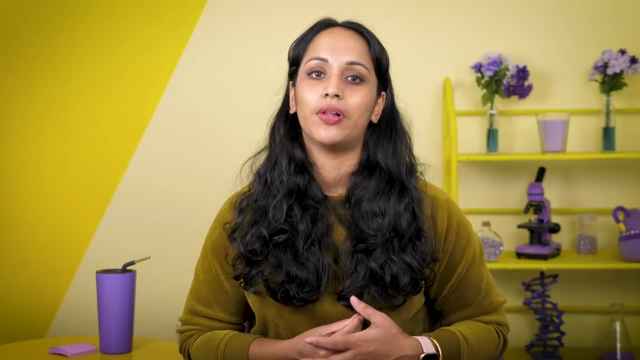 And even when it does, only one bromine atom adds and we keep the pi bonds. It turns out that the electron distribution in benzene actually makes it less nucleophilic than a simple alkene, thanks to conjugation, Essentially in a molecule with alternating double and single carbon-carbon bonds. 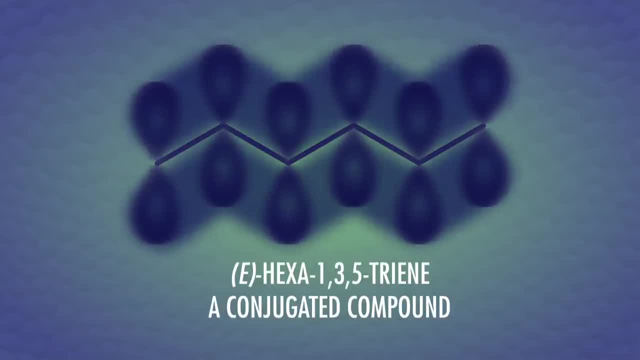 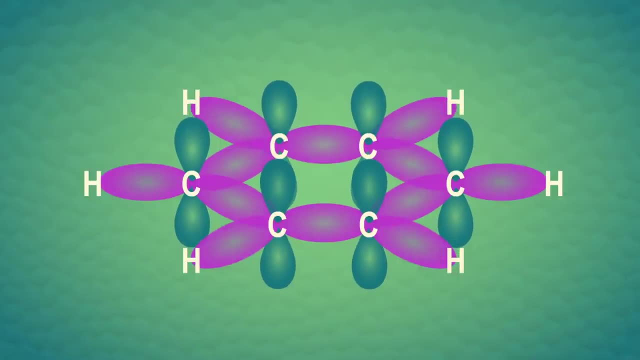 the p orbitals overlap, giving all of the bonds partial double-bond character. And because benzene is a ring, the p orbitals on each carbon atom align. We get something kind of like a hamburger – the pi bonds are the bread and the sigma. 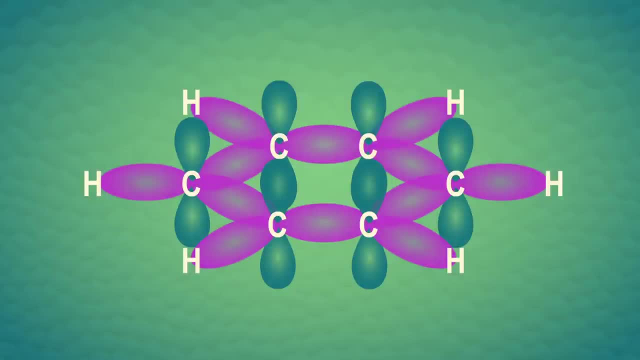 bonds are the meat. There are six pi electrons, one for each p orbital and they're evenly distributed around the ring. So we say the pi bonds in benzene are delocalized. Overall a pi bond in benzene has lower electron density than in an atom. 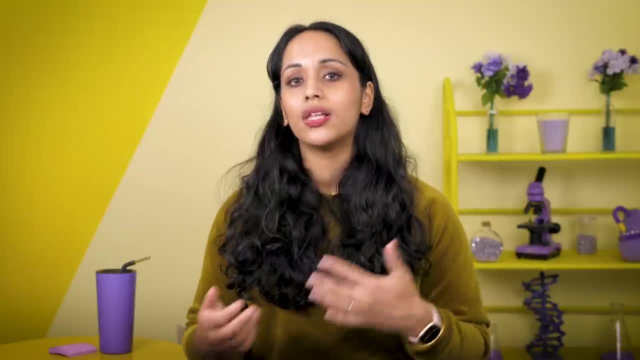 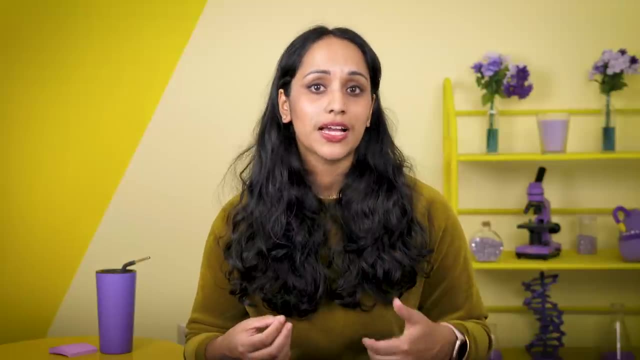 That's why it's called a carbonyl. It's also called a carbonyl. It's a combination of a benzene and an alkene, where electrons are localized between two carbon atoms, And this explains the lower reactivity. With delocalized electrons, benzene is less effective at polarizing other molecules. 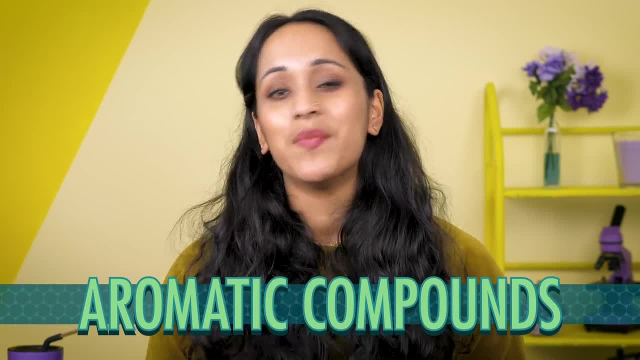 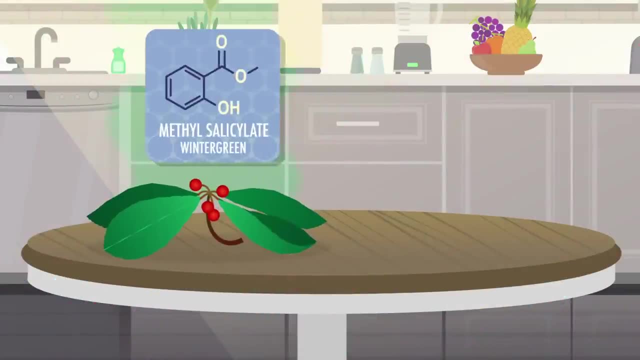 Benzene is part of a family of aromatic compounds. The name comes from the fact that many of these substances were first extracted from smelly stuff. For example, the smell of wintergreen leaves comes from methyl salicylate, while the smell of cinnamon comes from cinnamaldehyde. Besides their scents, aromatic compounds also have a smell. They're also known as aromatics. Aromatics all share four key characteristics. First, aromatics are cyclic: They all have a ring structure. Second, their rings are planar, which means they're flat. 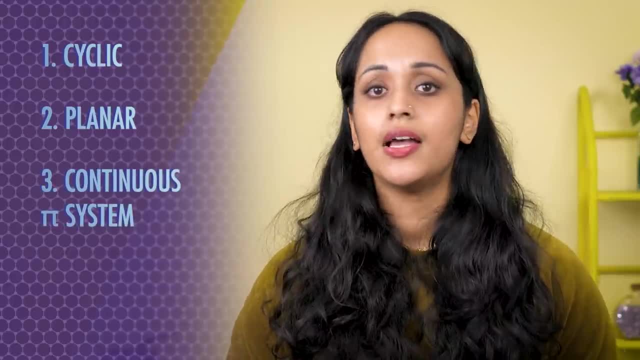 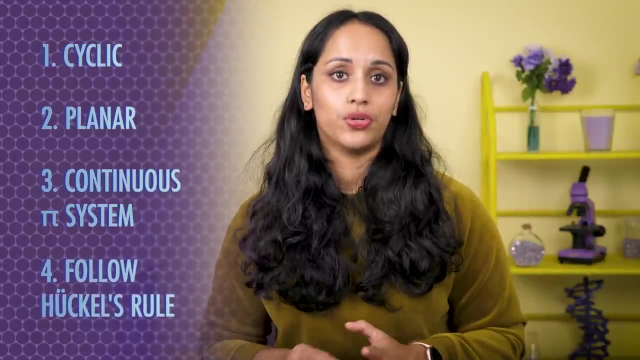 Third, they have conjugation throughout the entire ring, the smeared, continuous stretch of delocalized pi electrons we've been talking about. And finally, they follow Huckel's rule. This rule is named after German chemist and physicist Erich Huckel, who noticed that if 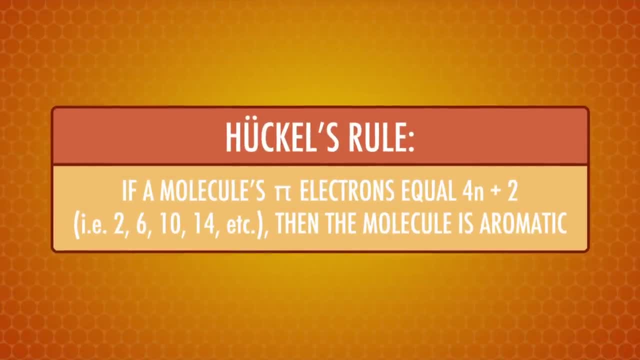 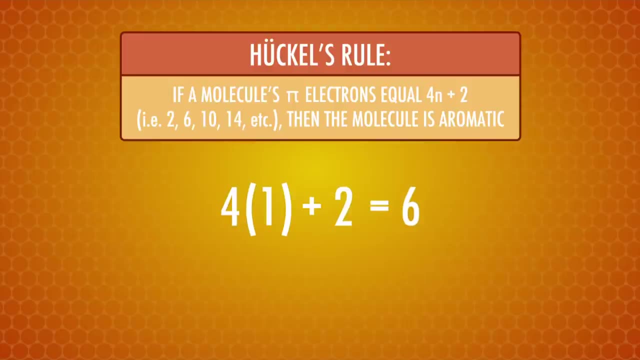 the number of pi electrons in a compound equals 4n plus 2, where n is an integral, then the compound is aromatic. For example, let's say n equals 1.. So 4 times 1 plus 2 equals 6 pi electrons. 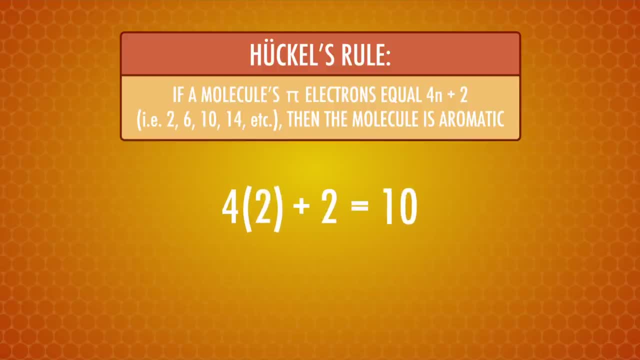 Benzene has 6 pi electrons and it's aromatic. And if n equals 2, we get 4 times 2 plus 2 equals 10 pi electrons. That works for naphthalene, which is also aromatic. By the way, if we drew naphthalene with circles in the middle of each ring, it sort of implies: 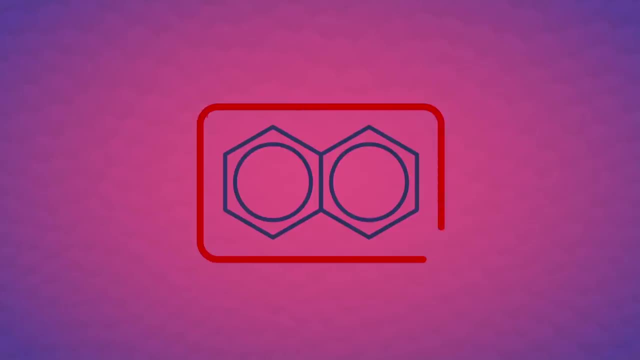 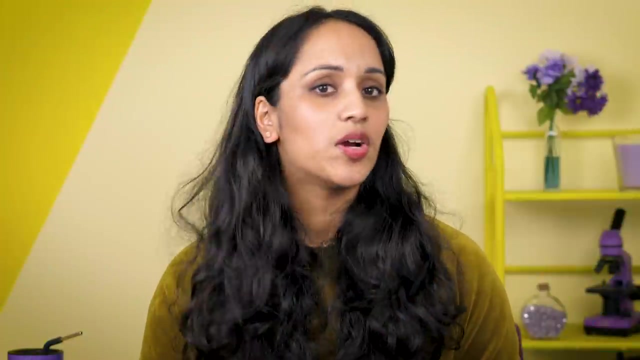 two pi bonds in the middle where the rings are joined, Which isn't the case. So this is not the case. This is why it's better to use the alternating bonds model when we're drawing polycyclics. Now, not all aromatic compounds are perfect. 6-carbon hexagons. 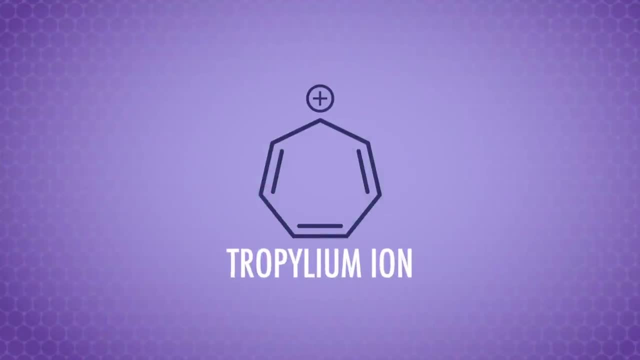 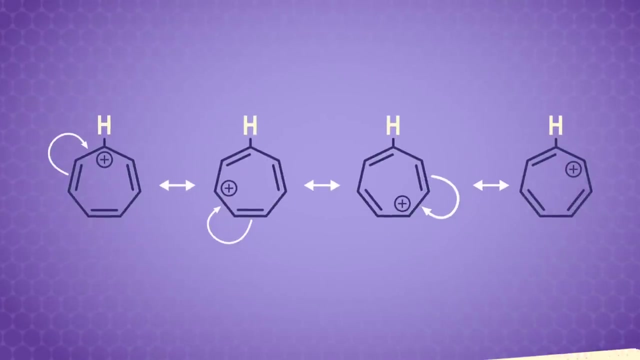 We see aromaticity in certain ions too. like a tropillium cation, a 7-membered ring with a positive charge. It has an empty p orbital and since we can draw resonance structures that delocalize the positive charge and the 6 pi electrons around the ring, the pi electron system is. 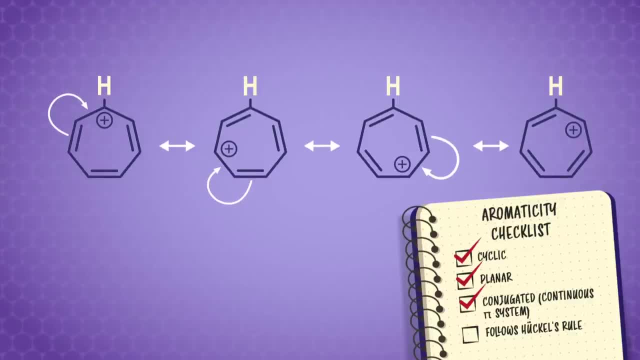 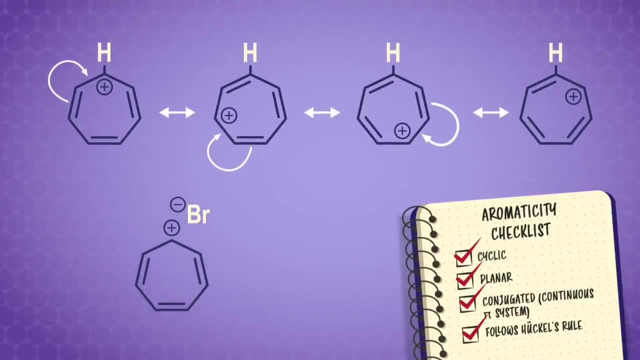 continuous. It's cyclic, planar conjugated and with those 6 pi electrons, like benzene, it follows Huckel's rule. It's aromatic, And tropillium salts, such as tropillium bromide, are remarkably stable. 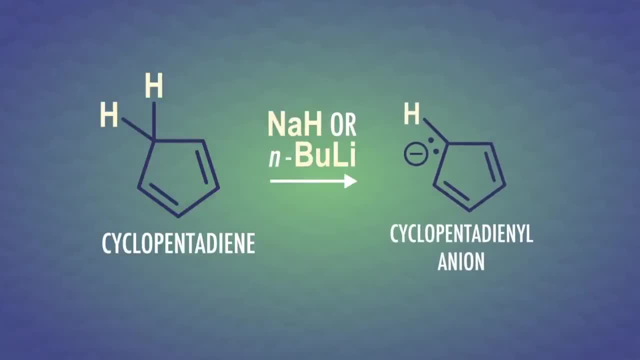 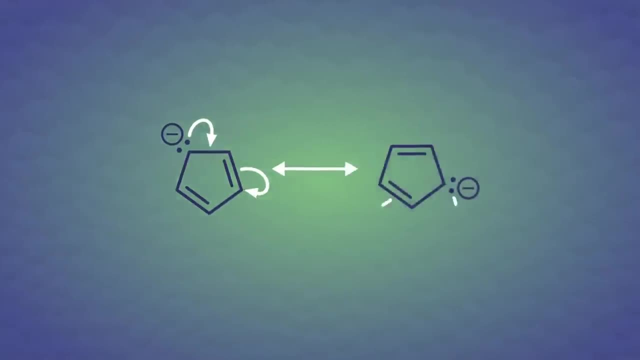 The cyclopentadienyl anion is an aromatic ion too. A strong base can deprotonate cyclopentadiene, putting a pair of electrons into a p orbital. The anion that results is cyclic, planar, has a continuous series of p orbitals, and 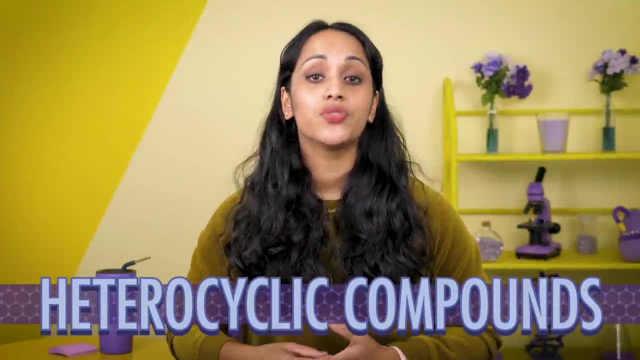 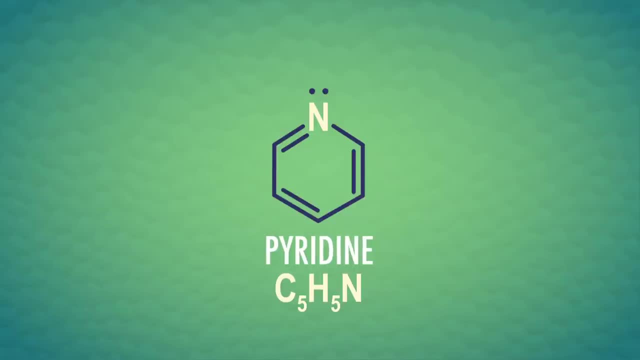 has 6 pi electrons. We also have heterocyclic compounds with aromaticity, which are rings that include an atom other than carbon. For example, pyridine is C5H5N – it's cyclic planar and has 6 delocalized pi electrons. 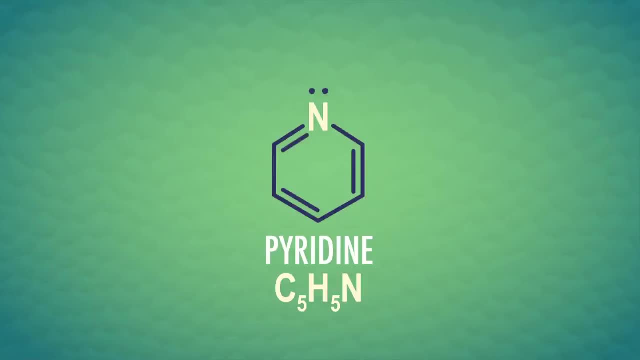 one of which is coming from the nitrogen, So it's aromatic. Nitrogen also has a lone pair in an sp2 orbital, but it's in the same plane as the sigma bonds – you know, the meat part of the molecule burger. 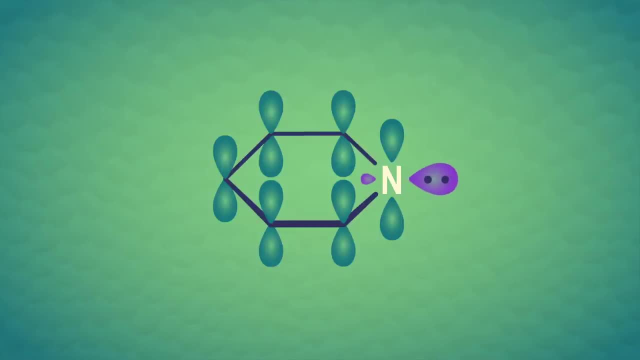 And because of the trigonal planar geometry, the lone pair of electrons can't be delocalized into the ring or burger bun and break Huckel's rule. In fact, this lone pair is available to accept a proton, which is why we'll see pyridine. 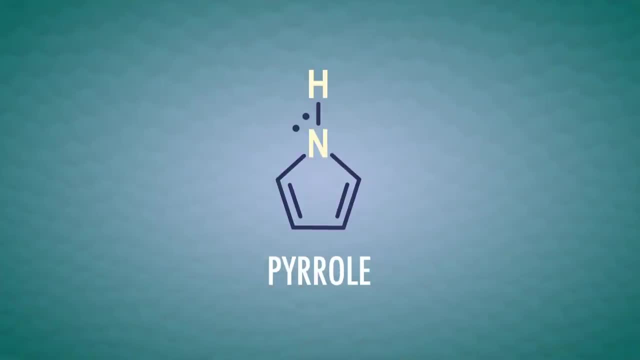 used as a base in some organic reactions. By contrast, the geometry of this heterocyclic compound, pyrrole, means that its nitrogen lone pair does contribute to the pi system, Just like the cyclopentadienyl anion. we end up with 6 delocalized pi electrons and pyrrole. 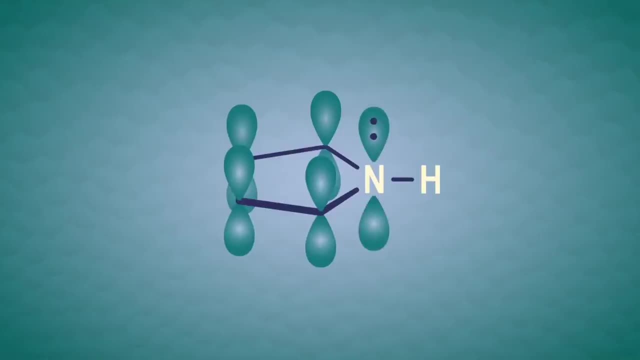 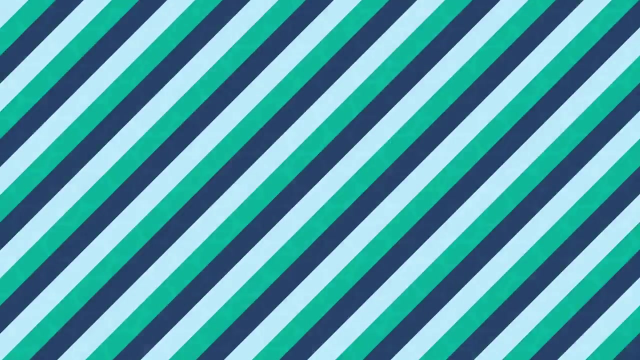 is aromatic too, But this lone pair is all tied up with its buddies. It's making an aromatic pi system. So pyrrole can't be used as a base like pyridine. The same goes for furan, only there's an oxygen instead of a nitrogen. 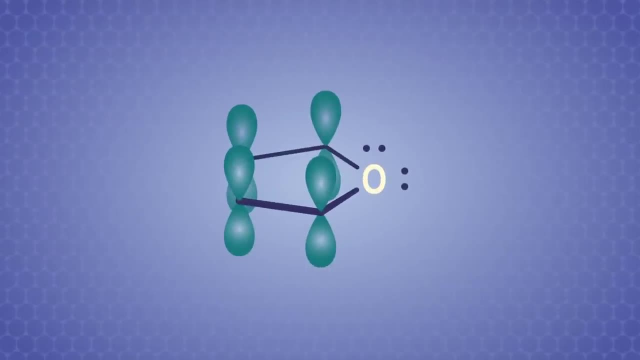 Because of this compound's geometry, only one of the oxygen lone pairs is incorporated into the ring system, So we've still got 6 delocalized pi electrons, And this makes the oxygen atom, sp2, hybridized. So far we've looked at lots of aromatic compounds, but plenty of cyclic compounds. 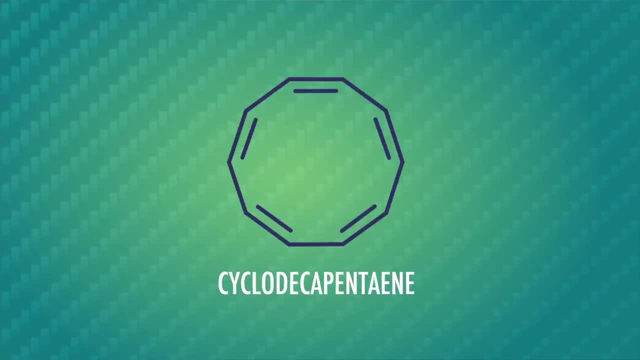 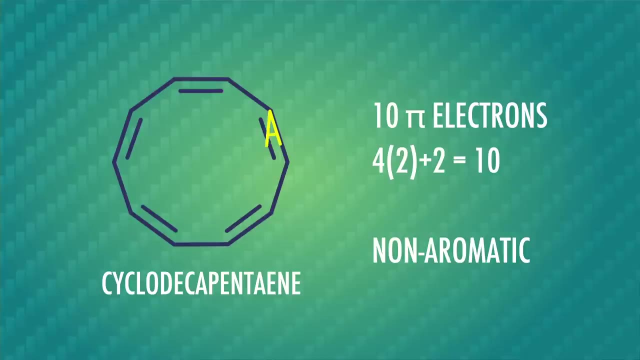 don't quite make the cut. For example…. Cyclodecapentaene follows Huckel's rule with 10 pi electrons, But it's not aromatic. If it were planar, a 10-membered ring would have 144-degree angles, which is much larger. 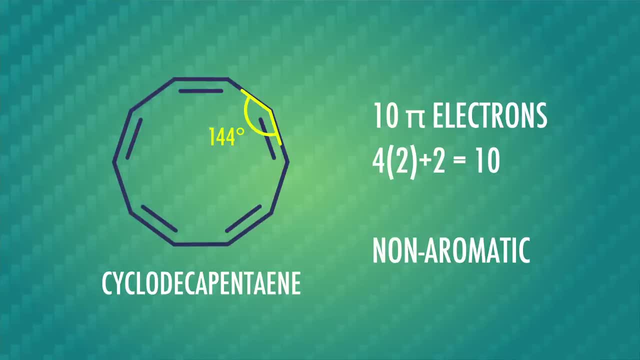 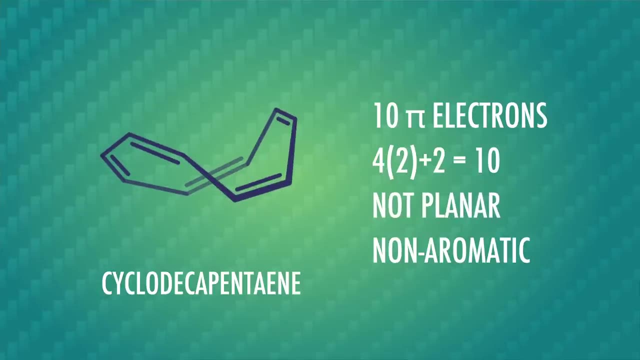 than the comfy 120-degree angles of sp2 hybridized carbons. So this ring puckers to become non-planar, breaking the overlap between the p orbitals. No conjugation, no aromaticity. sorry, There are also some cyclic planar conjugated compounds that don't make the cut. 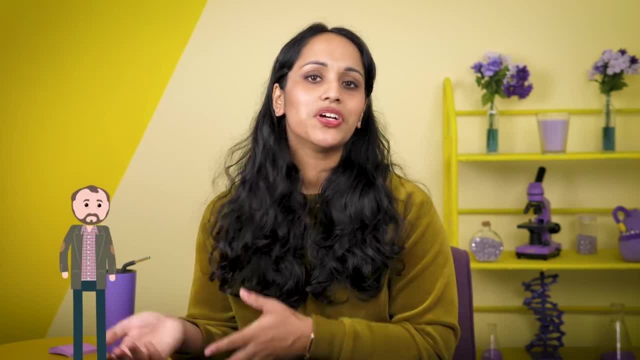 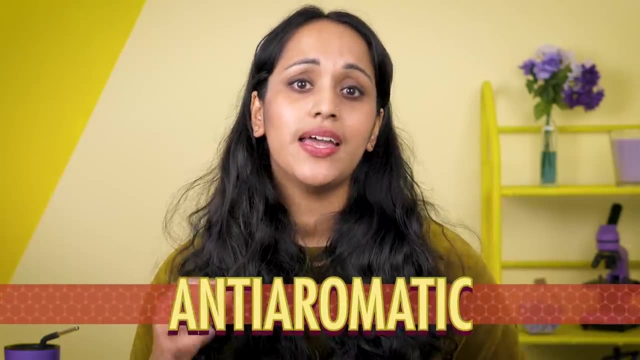 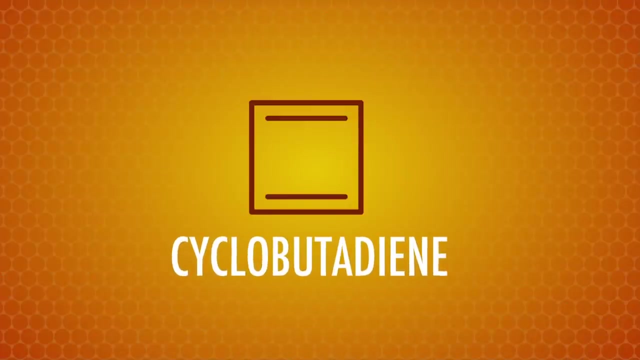 They look good at first, but then you realize something is a bit off, like creepy alien clones. These are anti-aromatic compounds and tend to be very unstable with 4n electrons where n is still an integer. One anti-aromatic example is cyclobutadiene with 4 pi electrons. 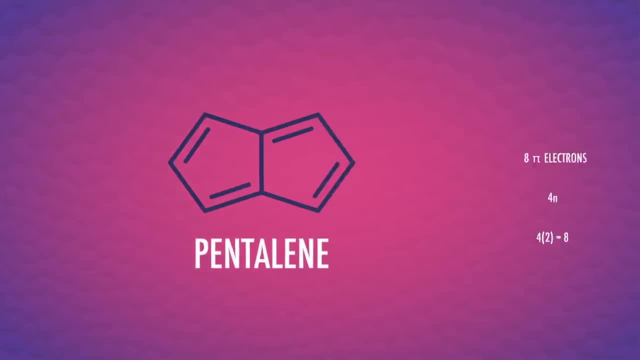 Or there's pentelene, which looks a little bit like naphthalene but it has 8 pi electrons. But while this 8-membered cyclooctatetraene gets close to being anti-aromatic, it's not. 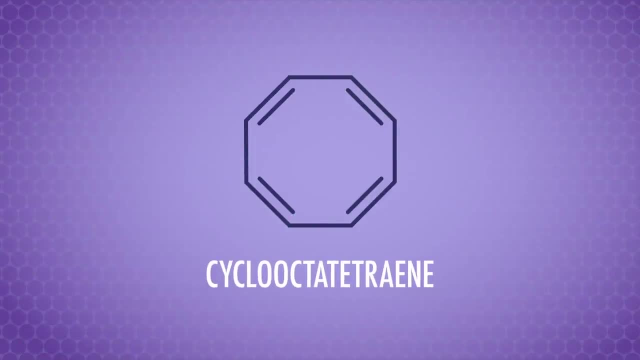 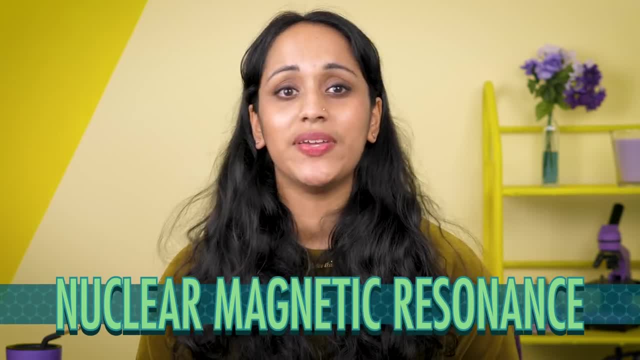 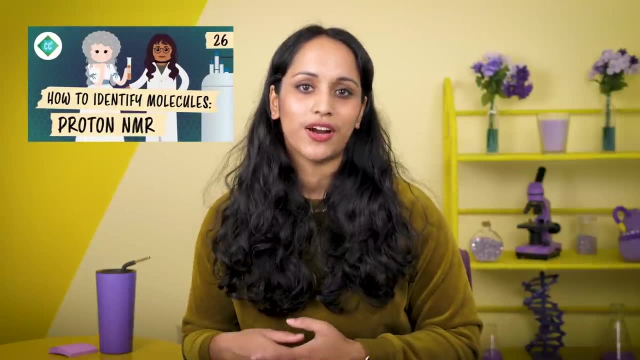 In the lab, when you have some stuff in a flask, nuclear magnetic resonance can be a great way to find out whether a molecule has aromaticity. We met NMR in episode 26,, so rewatch that video if you want a refresher. 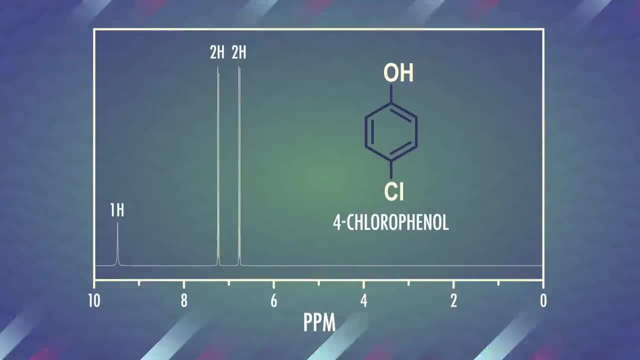 But we'll try to ease back into reading spectra with an example. This is the proton NMR spectrum of 4-chlorophenol, which is a benzene ring with a Cl on it on one side and an OH at the other. 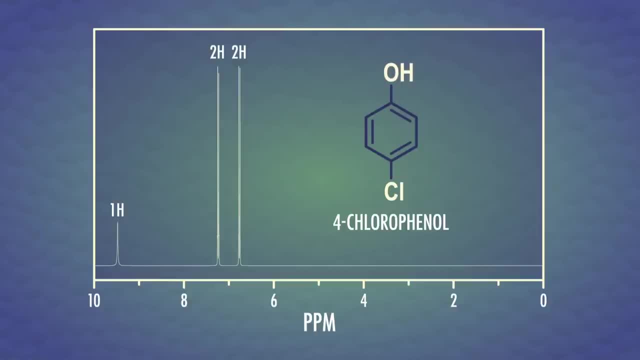 There are three peaks here and remember each peak represents a proton or group of protons in a molecule. We can see that the peak at 9.5 ppm with an integral of 1 is the one OH proton on the phenol. 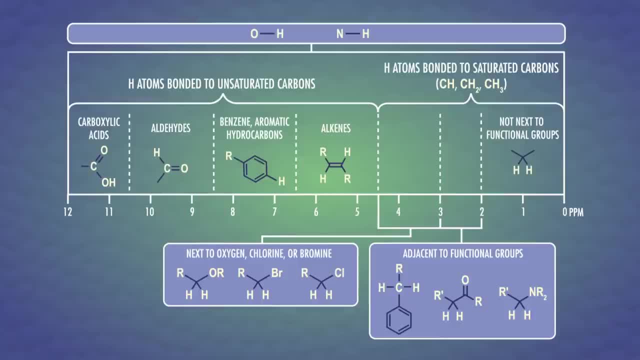 Easy Now. the protons attached to a benzene ring are a little less downfield – they're between 8.5 and 6.5 ppm or so. Because of the way the pi orbital system interacts with the magnetic field, these protons are quite deshielded. 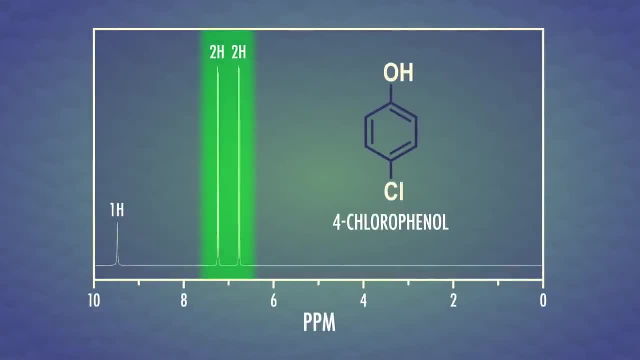 And there are two peaks in this region, each with an integral of 2, which represents two protons. But looking at the structure of 4-chlorophenol, we can see there are four protons on the aromatic ring. 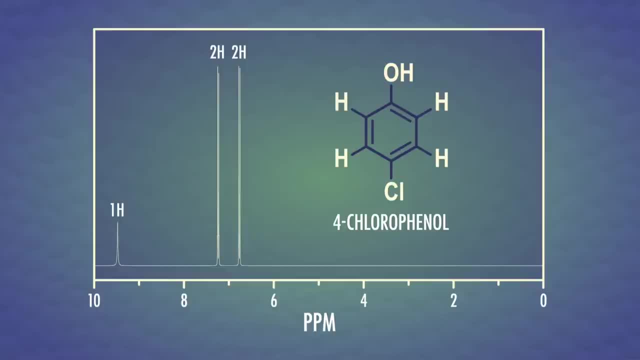 We only see two peaks in the NMR spectrum because this compound is symmetrical. If you put a mirror through the middle of the ring, the protons are effectively the same on both sides. In other words, they're chemically equivalent to each other. 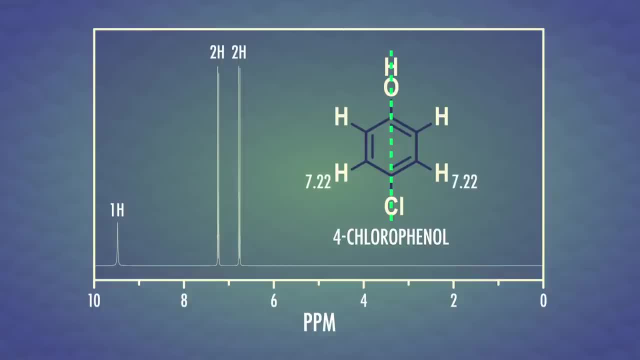 Specifically, the two protons near the chlorine are equivalent to each other, and so are the two protons near the hydroxide. The chlorine and hydroxide have slightly different shielding effects, which is why we see two peaks, each with an integral of 2.. 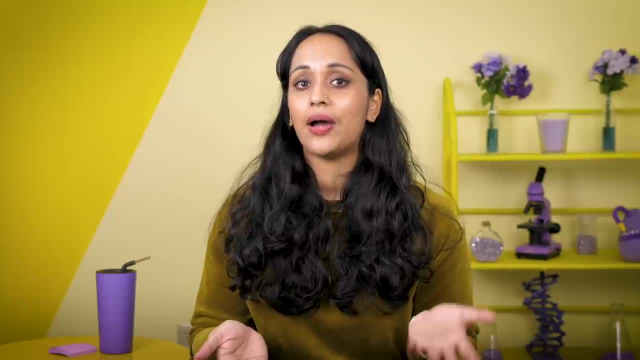 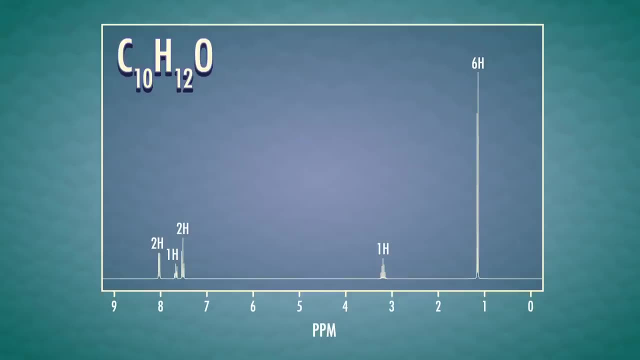 Now that we've done some practice, let's try to figure out an aromatic compound based on the proton NMR spectrum. We know its formula – C10H12O, And we have an IR spectrum with a carbonyl stretch, So we know it's an aldehyde or ketone. 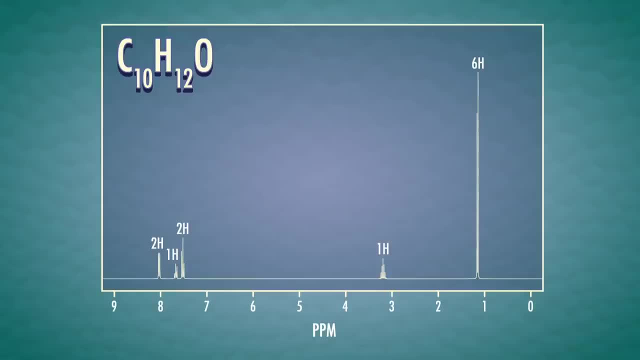 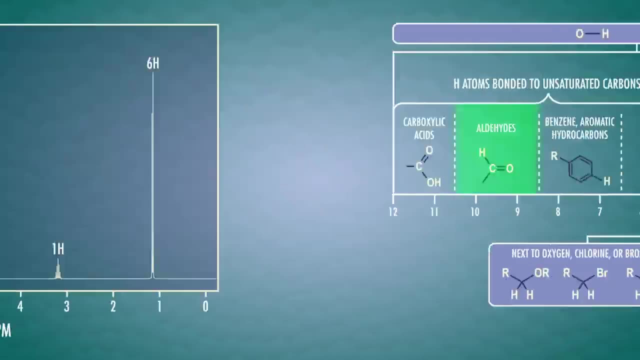 So let's dig into these NMR peaks and integrals. By looking at our NMR table, we know that an aldehyde proton would appear between 9 and 10 ppm. There's no peak there, so it looks like our mystery compound is a ketone. 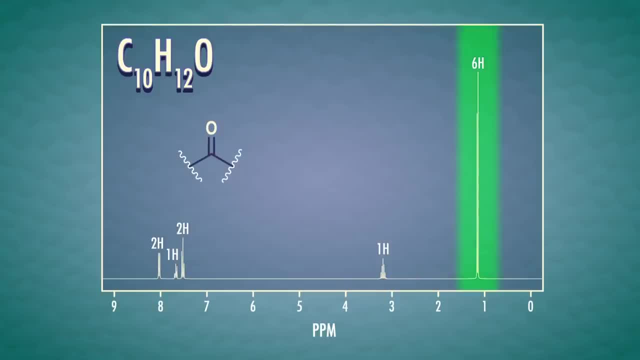 Next let's look at the huge peak over on the right with an integral of 6.. That's weird, right? One carbon can't have six protons attached, But we know that chemically equivalent protons can all combine into one peak. 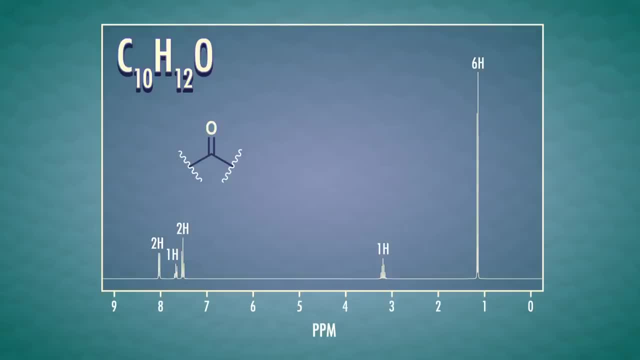 So there has to be some symmetry going on here and we just need to puzzle it out. Six hydrogen atoms can come from the protons on two chemically equivalent methyl groups which could be attached to the same atom. Let's try a carbon. 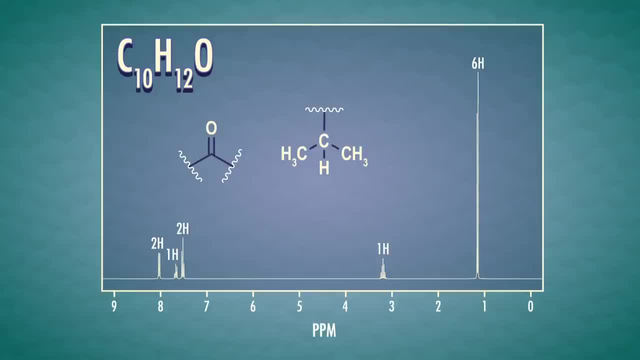 So here we have an isopropyl group with six chemically equivalent protons, because there's a line of symmetry through the middle. If we look a little downfield, there's a peak at 3.25 ppm with an integral of 1..